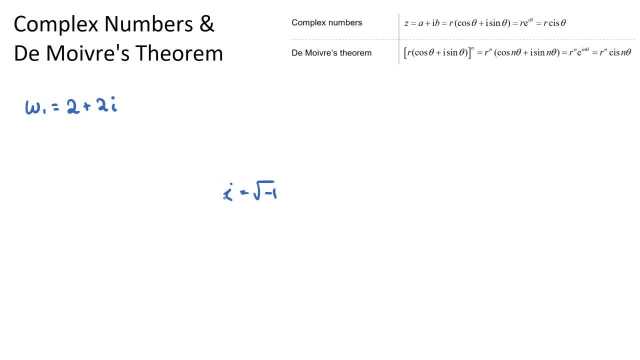 this in this topic of complex numbers, where we have real and imaginary numbers. Okay, so we can see an i in our number here and how we can. how we can view this is there's a real component of 2 and an imaginary component of 2 as well, So it's 2 plus 2i, where the first 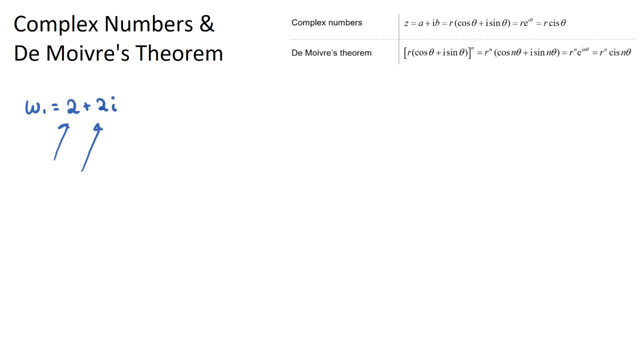 number is the real and the second is the imaginary component, And we can write our complex numbers in a few different formats. So in this format here is the same as this one up here. This is called Cartesian form. So Cartesian form is when you have a plus ib And a very important concept that 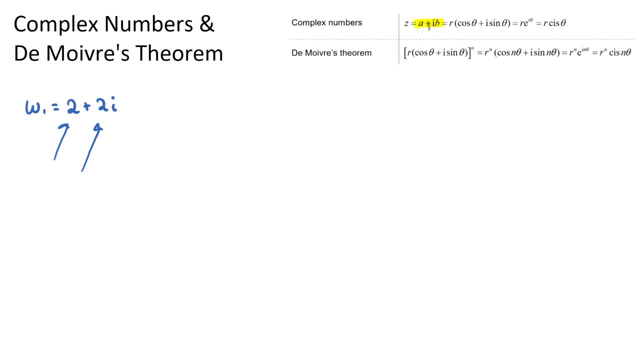 we need to know is how to convert from Cartesian form to modulus argument form, which is this one: r cosθ plus i sinθ, And that's actually the same as this one here. This r cisθ- Cis is just a short version of writing cos plus i sin. So if you ever see cis, that's just the same as cosθ. 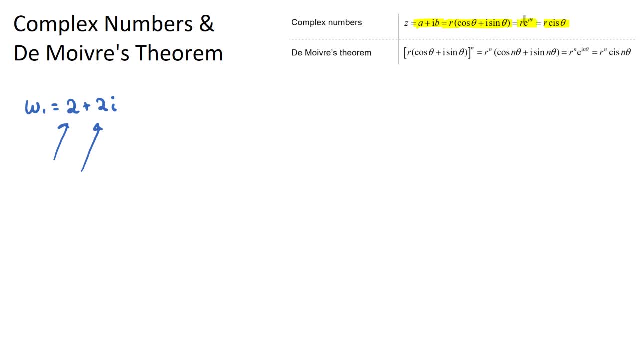 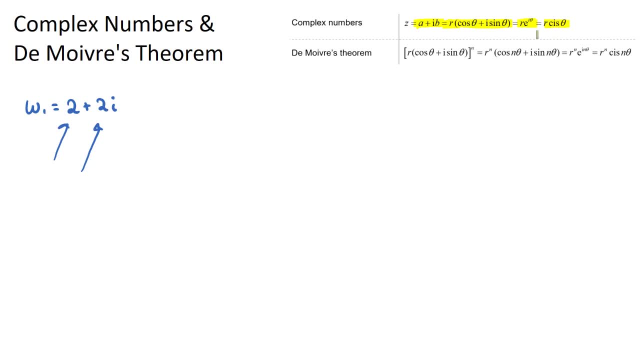 a complex number, but not as commonly seen as the other two. Okay, so if we have our complex number here in Cartesian form, we can actually draw where this number is on a axis, And in this topic of complex numbers, this is called an Argand diagram. Argand diagram where our vertical axis is the. 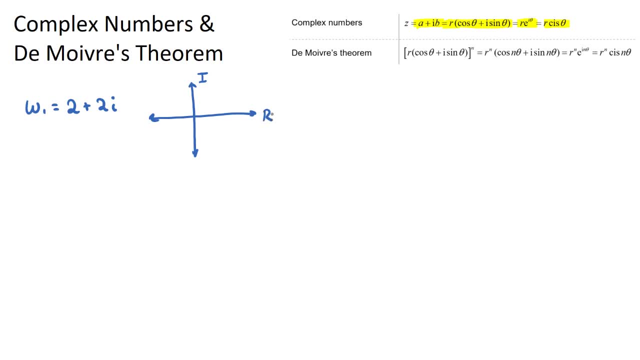 imaginary and our horizontal is the real. So we can plot where our number is here because it has a real component. So we have an imaginary component of positive 2, and an imaginary component of positive 2.. So our number will be here on our Argand diagram. And this is currently in Cartesian form. If we wanted to write it in modulus, argument form, what those two words mean, modulus means the size, the length. So if we picture this, this complex number, as being this line here, the modulus will be the length of this number. And you may have spotted. 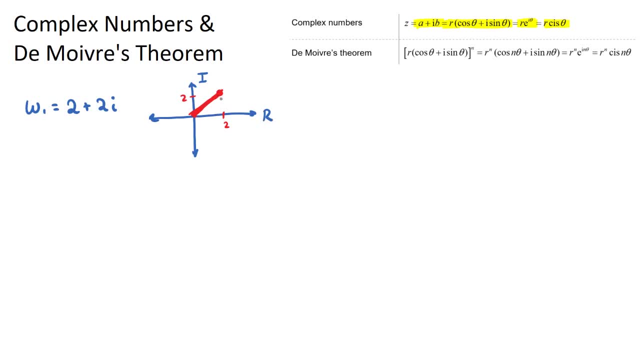 or you may have seen in a textbook, the length of a diagonal line. we know we can just use Pythagoras with the two components, with the x and y component or the real and imaginary component And the argument. so the modulus is the length, the argument is the angle that our complex number 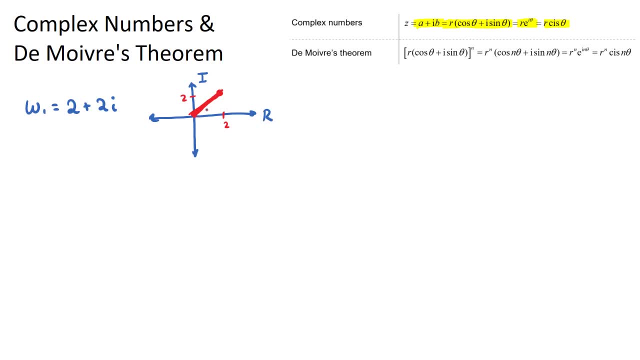 makes to the positive x-axis. So it'll be this one here. That's the modulus, that's the argument of a complex number. So let's convert our complex number here into a modulus argument form. The modulus we express as w1, with these absolute value signs around it. This is the 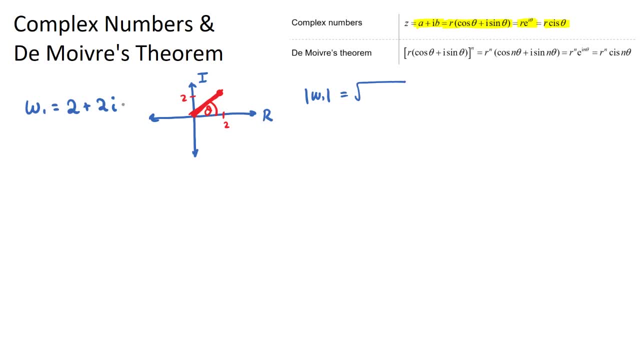 modulus And it's just going to be Pythagoras. It's the square root of each of the components squared. So 2 squared plus, and the imaginary component here is positive 2.. So plus 2 squared Now, this will be the square root of 4 plus 4, which is 8.. And this is just 2 root 2.. 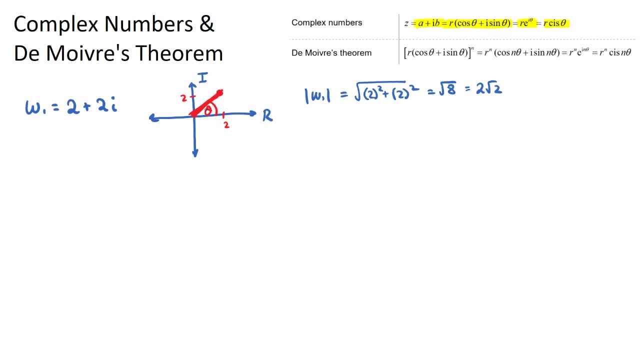 So this will be the modulus and that is the length of this line. here Now the argument theta. because we know the horizontal and the vertical component of our diagonal line, that's the opposite and the adjacent, we can use the tan to the negative 1 of opposite over adjacent. 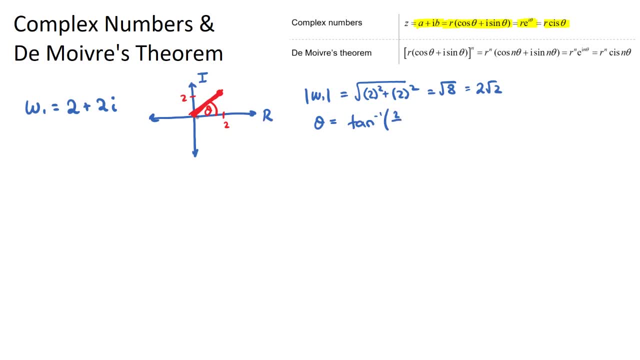 or the imaginary component over the real component. And that's how we find our argument for these complex numbers in Cartesian form. Now, tan to the negative 1 of 2 over 2, that's just tan to the negative 1 of 1.. And if we remember our trigonometric ratios- 1, 1, root 2, pi on 4, we know that tan of pi on 4. 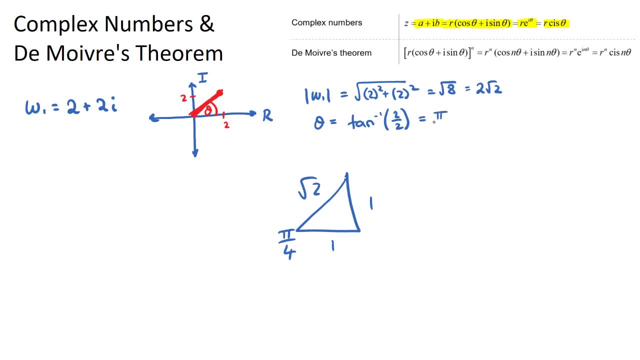 is 1.. So this angle here will be pi on 4.. Okay, So we've found our number here, So we can write w1 as 2 root 2 cis of pi on 4.. You could put the longer version and put 2 root 2 cos. 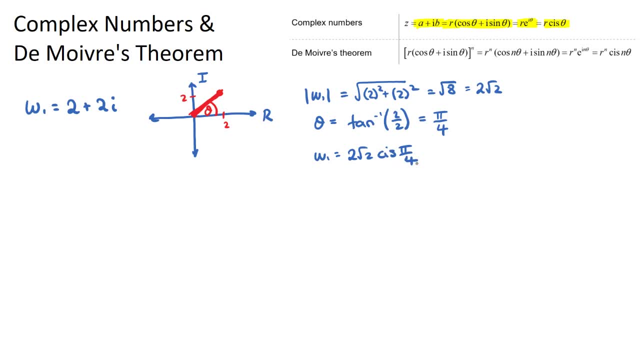 4 plus i sine palm 4, but this is just a shortened version, okay. so this is a very important key concept: knowing how to convert a complex number from cartesian form to modulus argument form. now, if i gave you another complex number, w2, and i'm going to give this to you, uh, straight away. 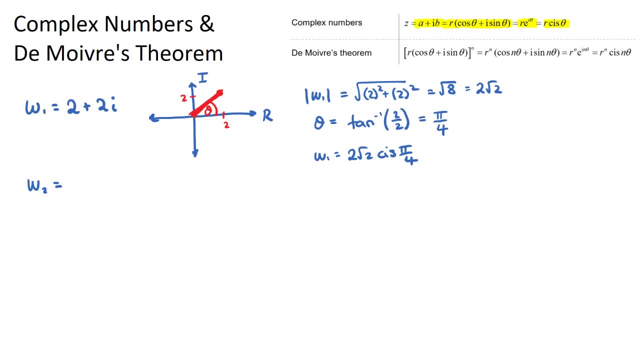 in modulus argument form. if it was root 2, cis 3, pi on 4, what some common ib questions often ask is, they'll say a new complex number, z. this is w1 multiplied by w2. it's the multiplication of two complex numbers. and if we have our complex numbers in modulus argument form, which we have, 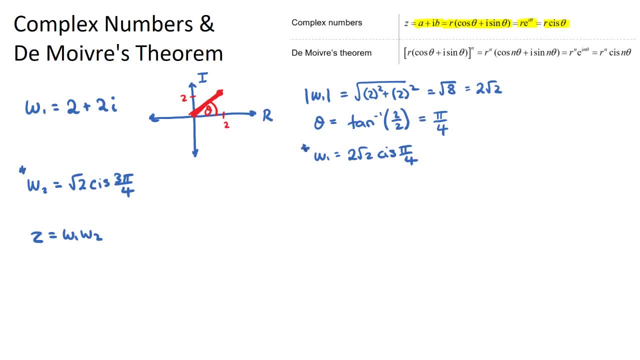 here, here and here there is a formula to to multiply two complex numbers. we just simply multiply the, the moduluses or the moduli of the two complex numbers. so 2 root 2 multiplied by root 2, and this will be 2 times and 2, so it'll be 4, and then we write cis and then we add the two. 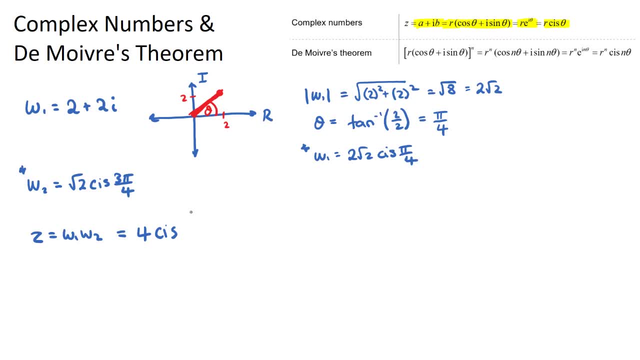 arguments. so 3 pi on 4 plus pi on 4 is 4 pi on 4, which is just pi. and i've done this one on purpose, because this is an interesting complex number. z here for cis pi, because we can actually get a simplified answer for what this is. 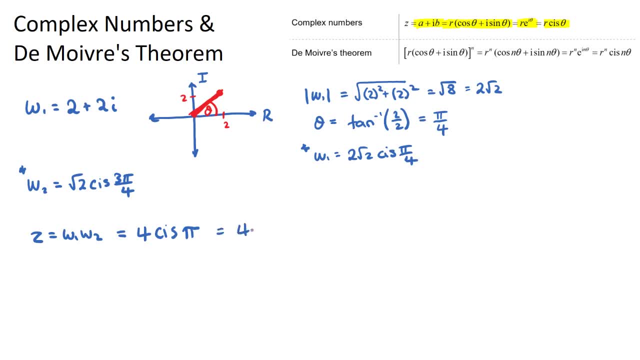 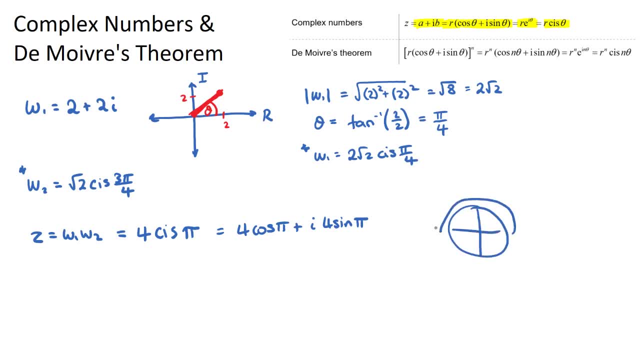 sign of pi all the way over at pi. here sine is the, the height, and sine of pi is zero. so if sine of pi is zero, 4 times 0 is 0. therefore there is no imaginary component to our complex number z. we will just have a real component. and cos of pi is negative 1, so it'll be negative 4. so the complex 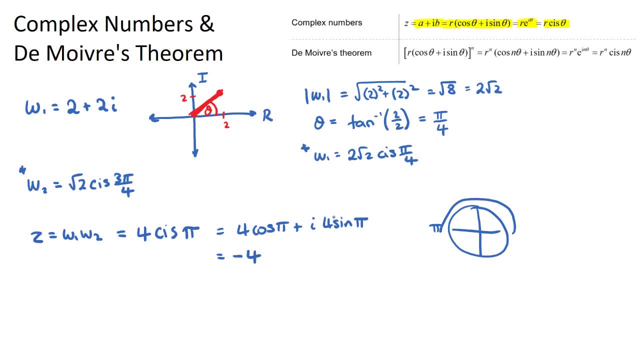 number z just has a real component here of negative 4, and there is no imaginary components. So have a look. Be on the lookout for complex numbers that only have an imaginary and non-real, or just a real and no imaginary, because they do appear very often in IV questions. Okay, Now, lastly, I want to look at De Moivre's. 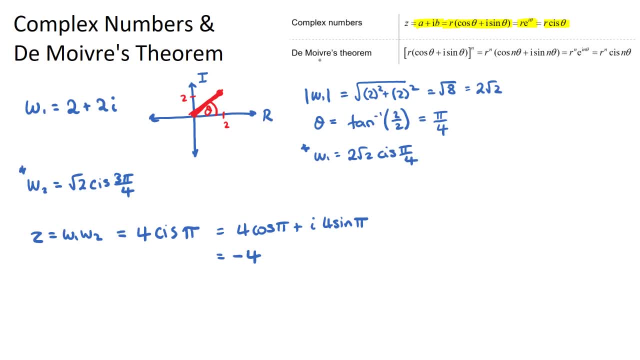 theorem. So De Moivre's theorem helps us raise complex numbers to a power. So let's have a look at the formula here. If we have some complex number to the power of n, De Moivre's theorem tells us that we raise the modulus to the power of n, and then we multiply our argument by n. 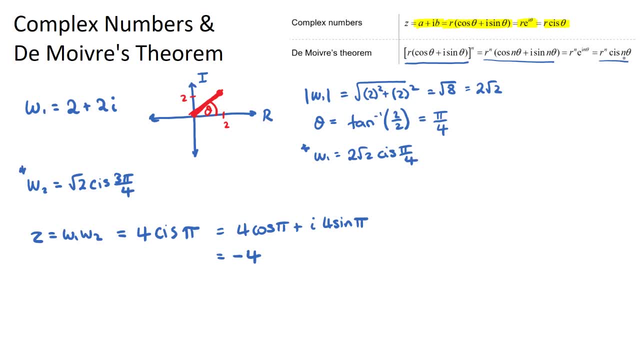 So that's how we get this form here. There's r to the n cis n theta. That's just the shortened version, and here is the polar form version as well. So a small example of that is: if I wanted to raise. 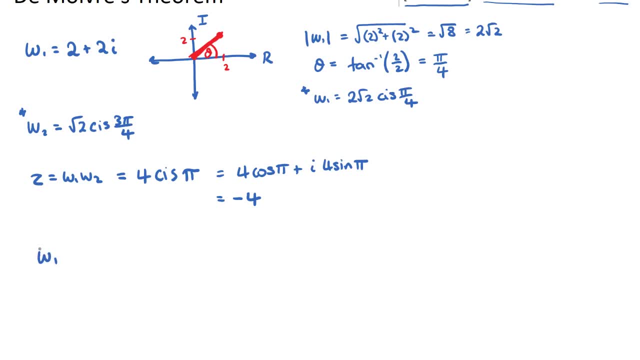 Let's say our first complex number, w1, to the power of 3.. If I wanted to raise it to the power of 3, what we need to do is we need to put it into, We need to put it into modulus argument. 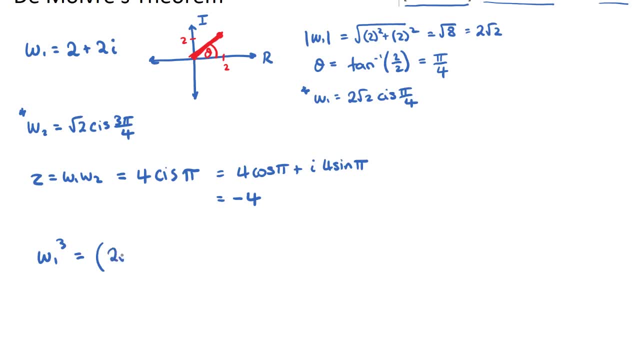 form first, which we have here. So we'll have 2 root 2, cis pi on 4, all to the power of 3, and then, by using De Moivre's theorem, we know that this is just 2 root 2 to the power of 3,. 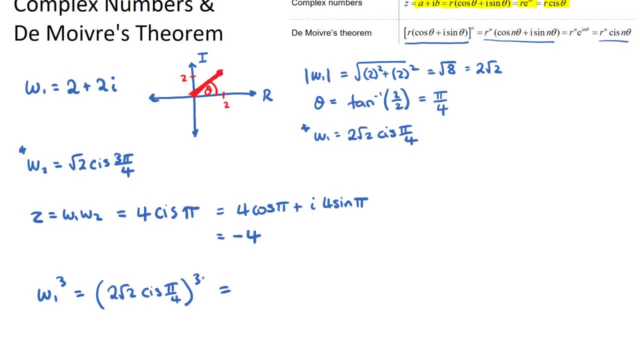 Now, that is 2 to the power of 3 and root 2 to the power of 3.. 2 to the power of 3 is 8.. Root 2 to the power of 3 is 2 root 2.. So we'll get 16 root 2, and then cis. 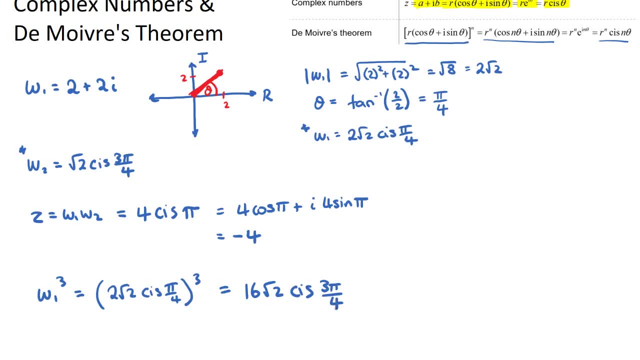 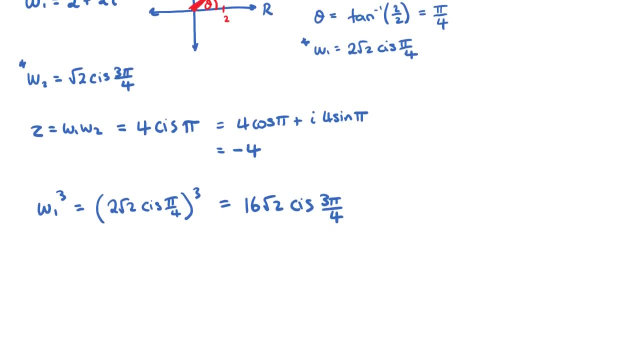 and this will become 3 pi on 4.. Okay, so that's how we use De Moivre's theorem and I'm just going to quickly show you and you might be able to practice some questions on this De Moivre's. 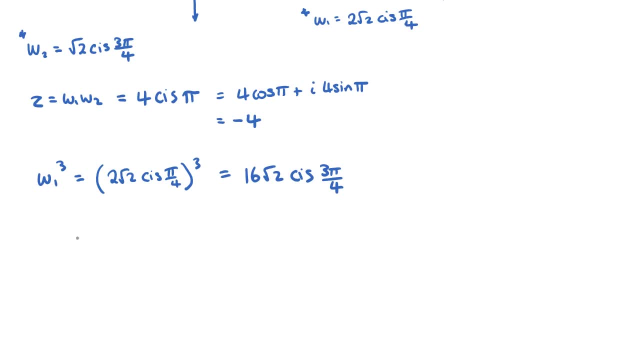 theorem is most popular in questions and it's very popular in questions and it's very popular where you want to find the roots of a complex number. and what a question might look like is they'll say: if z cubed is equal to 8i, where z is the roots of this complex number, 8i. 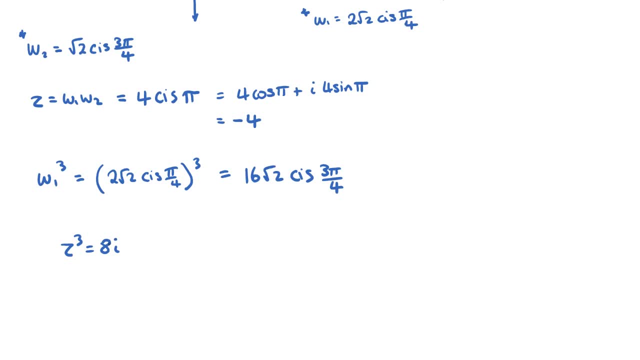 we know that we can turn 8i into a complex number in modulus argument form. This would become 8 cis pi on 2. This takes a bit of practice but we know that i doesn't have a real component. so that would be eight units directly up, and directly up will have.